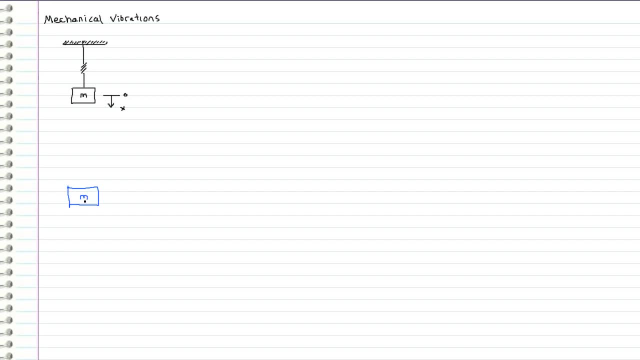 Here's our block, And now what kind of forces are acting on it? Well, it has mass. So we know that we're going to have gravity, So this is going to be a gravity force going downwards on it, And we also have a spring right here. So we're going to have a spring force also acting on this block. But before I draw the force on here, we need to pick a model for our spring. So typically, let's go ahead and just pick an easy model. That's typically how we model systems. The point is to simplify things. So 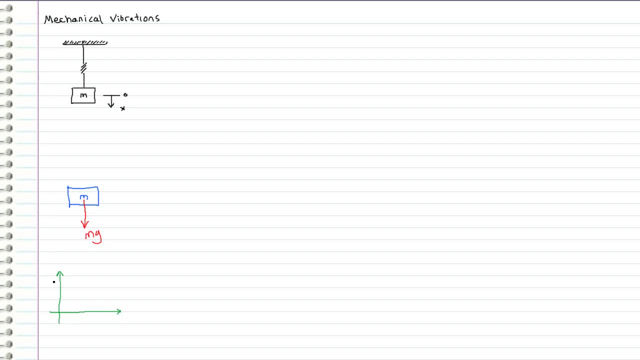 let's go ahead and pick a linear model for our spring. So all that means is that the spring force we'll call Fk. It varies linearly with the displacement of the spring from the relaxed length And it's going to have a slope of k. So this would be like the spring constant. 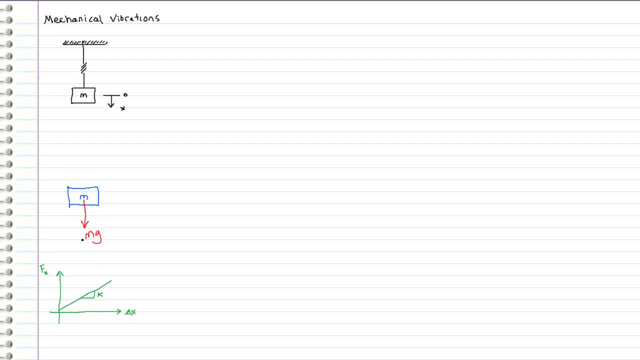 So all we are doing here is we chose to model the spring as a linear spring, meaning that the force varies linearly with the displacement. from the relaxed length And from Hooke's law, we know that this fk is going to equal negative. 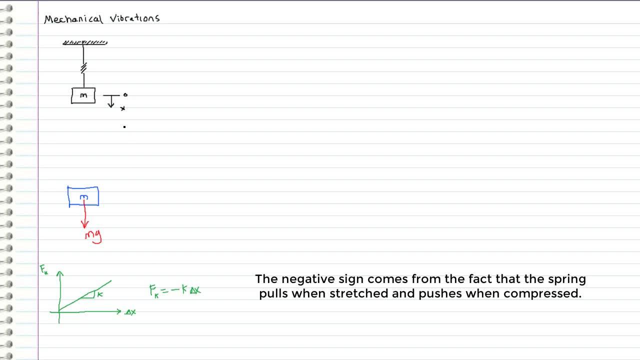 k times delta x. But since we have defined our coordinate system up here to be x equals zero at the relaxed length, we can actually just replace this with negative k times x. So this is our model for our linear spring and we can go ahead and now draw the force on it. So we have a 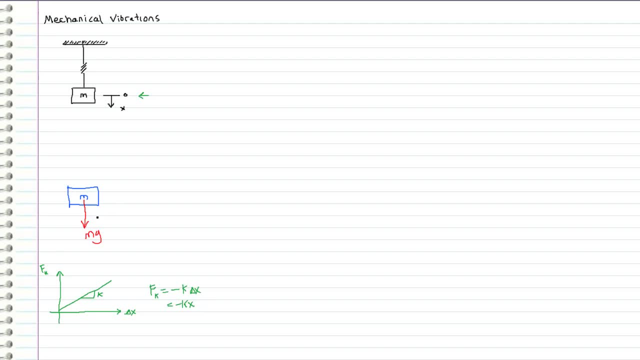 negative kx. so this force is going to act in the negative x direction. So I can just draw it pointing in this direction with a magnitude of k times x. Okay, so this is our free body diagram. We don't have any more forces acting on it at the moment. We will get there later. 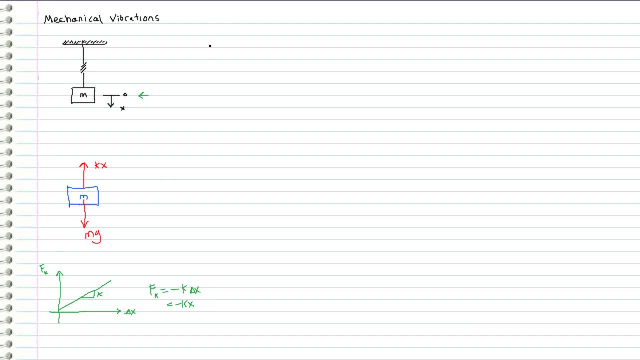 But so now let's go ahead and build our differential equation. So we call Newton's law: the sum of the forces is equal to mass times acceleration. So all we have to really do is just plug in for the sum of the forces, and that was the point of drawing our free body. 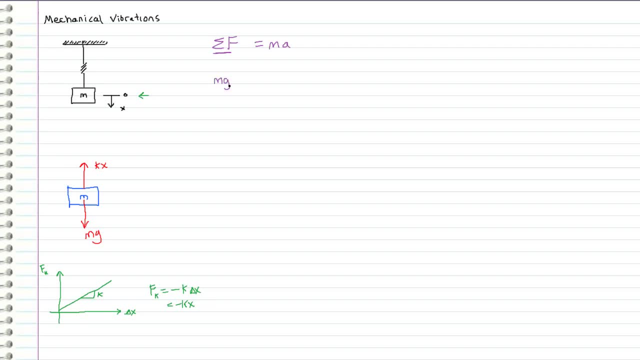 diagram. So let's go ahead and draw our free body diagram. So let's go ahead and draw our free diagram. So some of the forces we have m times g and then minus a k times x, and this is equal to m times a, And recall the acceleration. we can really just say that this is equal to m dv dt. 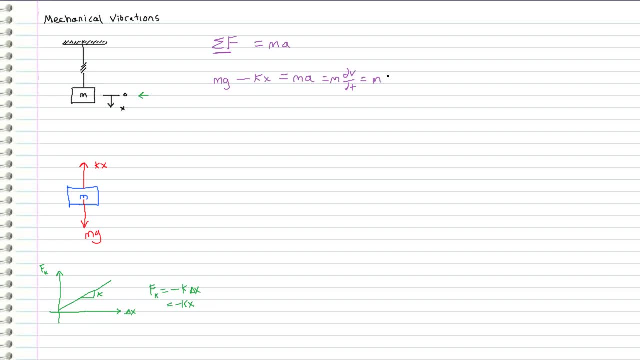 the rate of change of the velocity, or equivalently, m times d squared x dt squared, the derivative of the velocity. So we already see our differential equation emerging. We have some x double primes here. we have x right here and I'm just going to go ahead and rearrange. 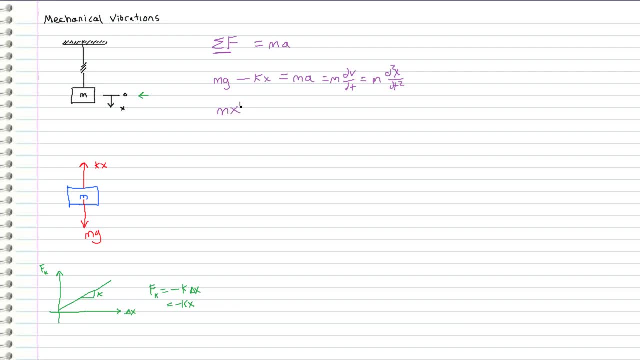 it to look like this: m times x, double prime. I'm going to drop this notation right here and just replace it with primes. We all know what that means. Plus k times x is equal to m times g. So what do we have here? Well, we have a constant coefficient. second order: non-homogeneous. 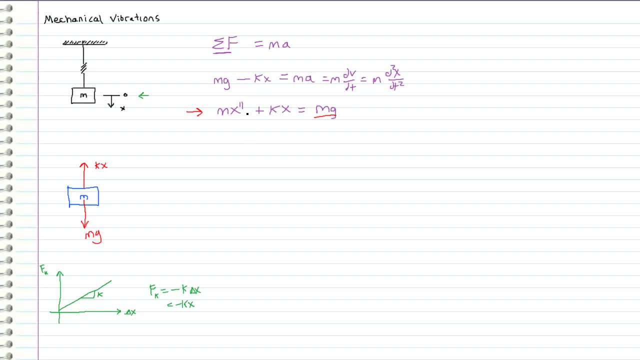 linear differential equation And we know exactly how to solve these. We've been learning this the past several videos with variation of parameters and undetermined coefficients. So in this one in particular, since we have a polynomial, a zero degree polynomial on the right hand side, we know that we can use undetermined coefficients. 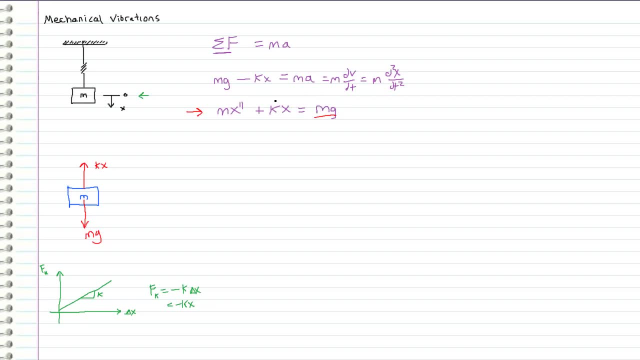 which is generally easier than variation of parameters. So that's probably how we will proceed in solving this kind of differential equation right here. But anyway, this differential equation serves as a model for this system, And if we solve this, what we get is a function x that describes the motion that this mass is going to have. So we're going to get a function x that describes the motion that this mass is going to have And if we solve this, what we get is a function x that describes the motion that this mass. 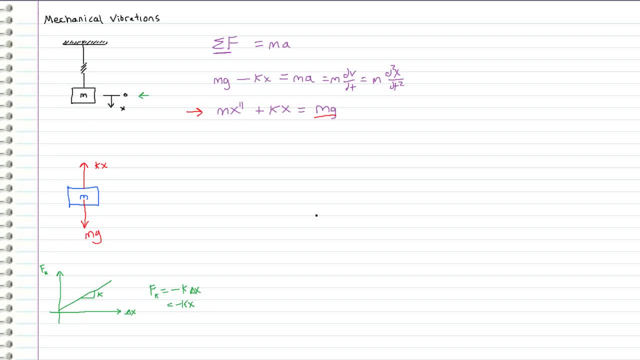 takes given certain loading conditions. We haven't specified those yet, But this is the differential equation that describes this system. Okay, now let's get a little bit crazy. Let's add some complexity to our model, Because typically in engineering, that's what we do: We start with. 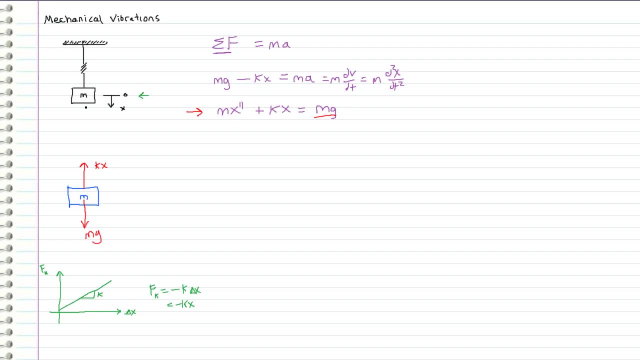 something very simple like this mass and spring system And then, depending on our application, we add layers of complexity to it and build that complexity into our models to give us more accurate representation of the model. So we're going to get a function x that describes the 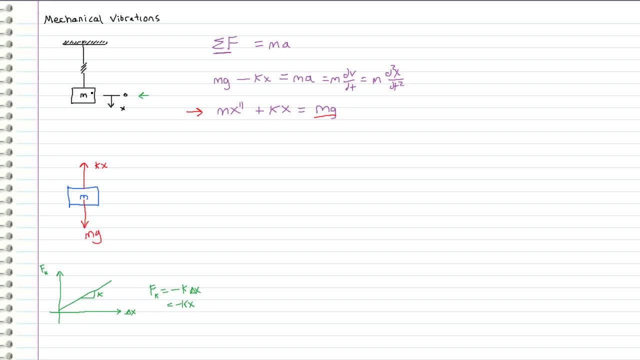 physical system that we are actually analyzing. So right now this model has no source of friction or dissipation of energy in it, And that's kind of unrealistic, because everything has friction and stuff like that. So let's go ahead and add a damper, a friction source, And I'm going to 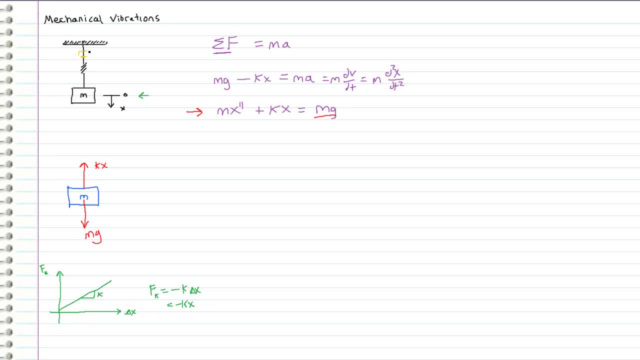 denote that, like this, I'm going to have this guy right here. So this is just representative of a damper. So now we need to find a model for this damper And typically, like I said earlier, we start with something very simple. 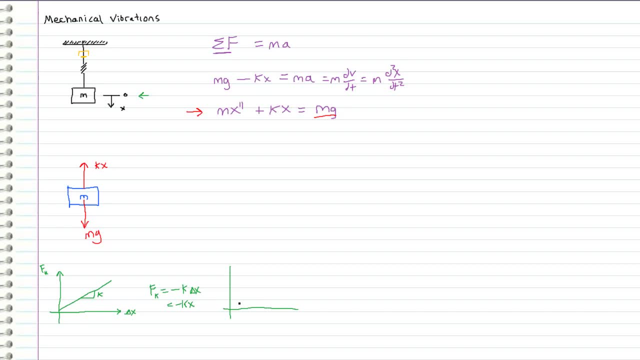 The easiest way to model a damper is a linear, viscous damper. So all that means is that, just like we did with the spring force, let's let this damper vary linearly. So the force of the damper- I'll just denote it Fd- is going to vary linearly with the velocity, And typically, 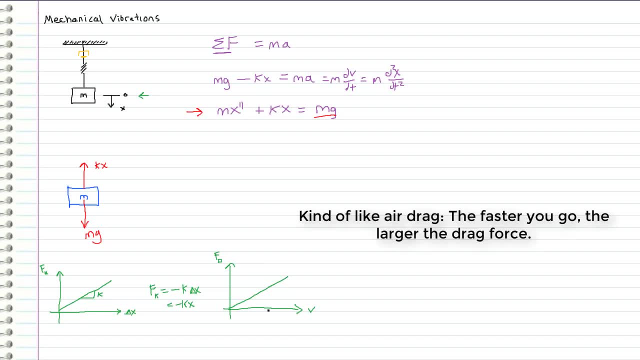 this is a good model for a viscous damper, with the velocity instead of the displacement, like a spring. and let's say the slope is c, so the damping coefficient is c. so again this means that fd is equal to negative c times the velocity, or equivalent negative c times x prime. and again this negative it comes from the fact that this is 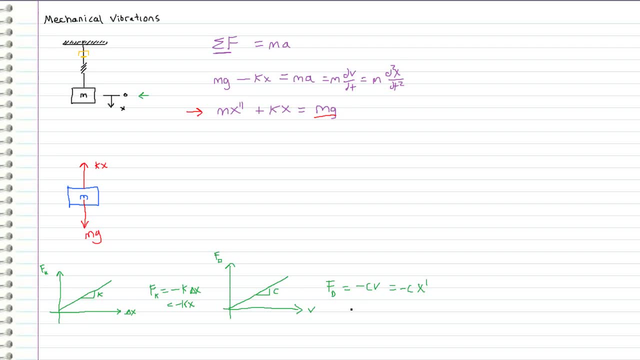 a friction force and friction always opposes the motion of which the the block is going to take. so the friction force is always a dissipative opposing force. that's why we have this negative. so we can add another force now to our free body diagram and i will call it c times v. okay, but we're 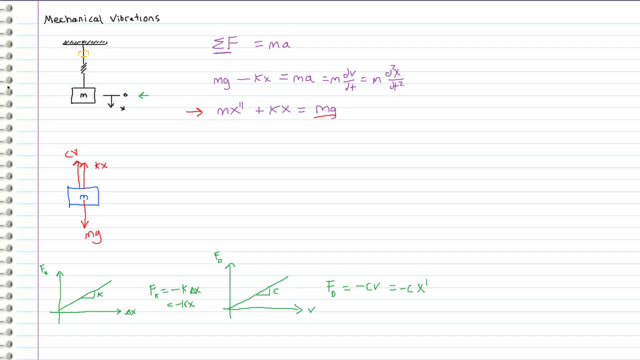 not done yet. let's add another layer of complexity here. let's say that that i'm standing over here, so here's me and i'm grabbing on this mass and i'm kind of pulling it and tugging it and stuff like that, pushing it, and basically what i'm going to be doing is i'm going to be. 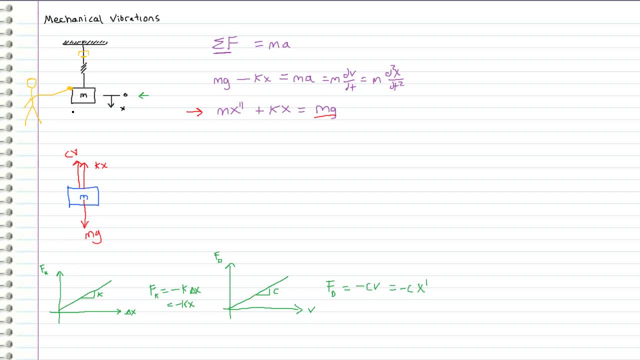 imparting a force on this block of mass m that's going to vary as a function of time. so i can represent that as a force on this block of mass m that varies with time. i'll call that f of t and again, i'm assuming that i'm only pushing and and lifting this block. 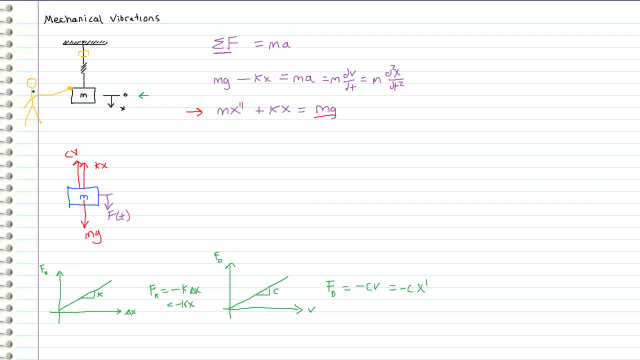 of mass m in the vertical direction along the x axis. there's no sideways action going on at all. so this is a a force that varies with time and now all we need to do is add the layers of complexity that we just added to this model back into our difference equation. so, instead of dealing with